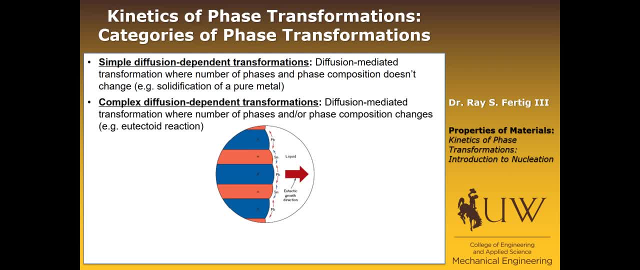 In this case, the number of phases and or the phase compositions are going to change, And an example of this would be a eutectoid reaction. What I'm showing you here is actually a eutectic reaction, But you can see the 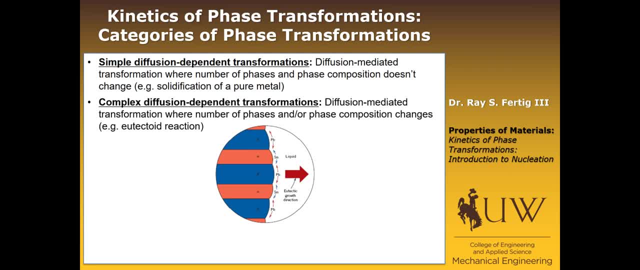 Eutectic growth direction. as the solid phase grows into the liquid phase, There's diffusion required from the liquid into one phase or away from another phase. Now, that would be a sort of one more level of complexity. And then, finally, there's a type of transformation called a diffusionless transformation, that proceeds without any diffusion. 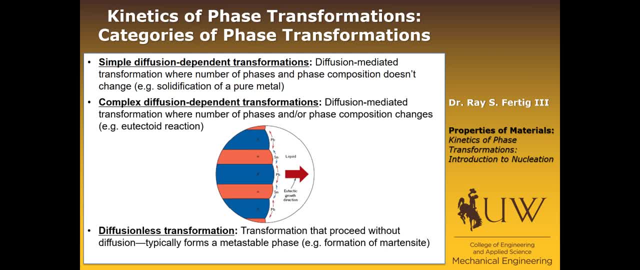 And this typically forms a metastable phase, And we're going to see this in the formation of martensite in steels. So those are the three types that are important to be aware of. We're going to talk today about a simple diffusion-dependent transformation, namely solidification of a pure metal in just a little bit. 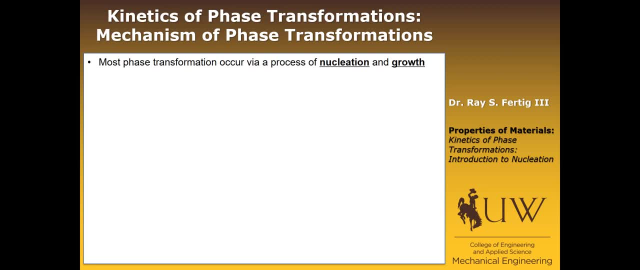 Most transformations, or most phase transformations that we're going to encounter occur via some process of nucleation and growth. And nucleation is exactly like it sounds: It's the formation of some small particles or nuclei, And those are. It's usually on the order of hundreds of atoms, of whatever new phase. 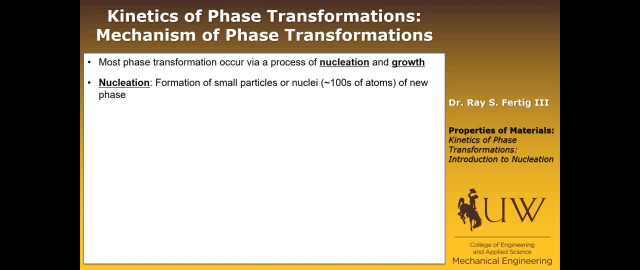 So in the case of the simple solidification that we're talking about, we're looking at, the new phase would be the solid phase. The growth phase is just once those particles or the nuclei form. they're going to increase in size until whatever the equilibrium phase amount that's required is obtained. 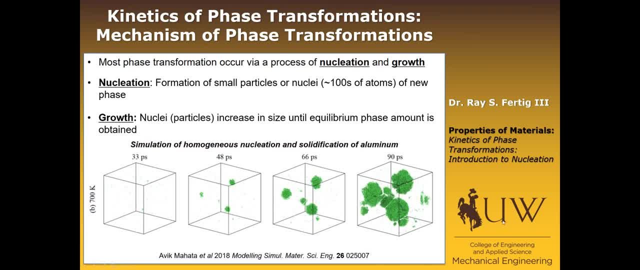 I'm showing you here a picture of of a simulated nucleation and growth process. This is for pure aluminum, and what you can see- and this is these- are times of the simulation. So 33 picoseconds, 48 picoseconds, 66 picoseconds and 90 picoseconds. 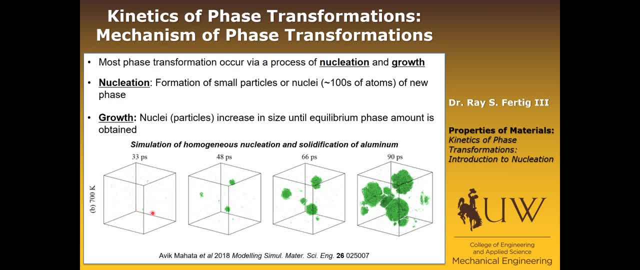 This is all done at 700 degrees Kelvin. But what you can see is in this early phase you can see some nuclei starting to form, these little green spots, And at some later time those nuclei have begun to grow. Here you go. 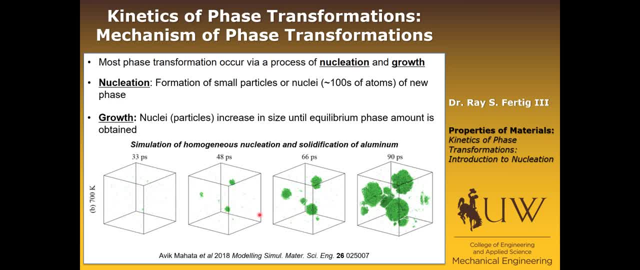 And some other nuclei now have started to form. Further on in time, the growing nuclei continue to grow and the new nuclei continue to grow, And then there are some right here, some new nuclei that form And that process continues until we get to a higher time and the growth continues and so does the nucleation. 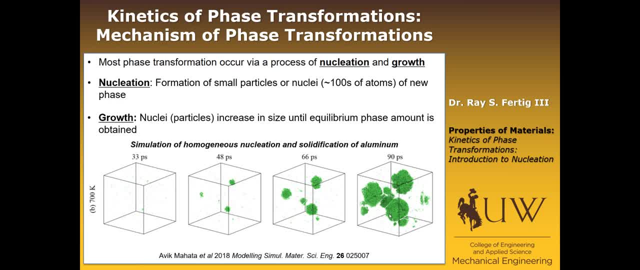 So be aware that nucleation and growth typically are occurring simultaneously. It's not one And then the other, except for at the particle phase, But in the process as a whole, nucleation is occurring at the same time that growth is occurring in other nuclei. 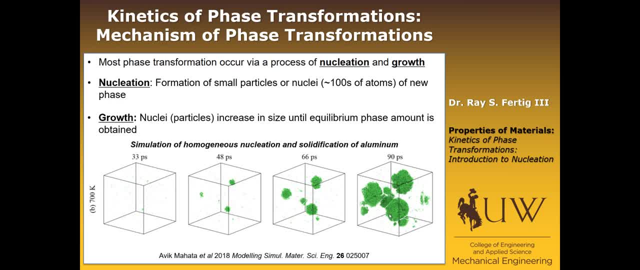 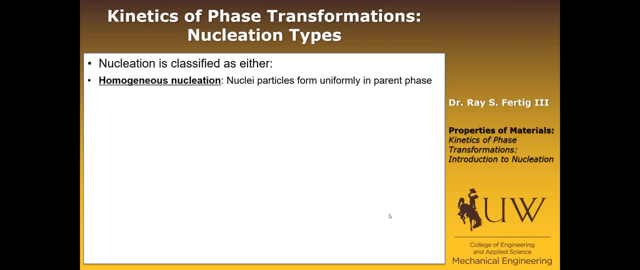 So those are important concepts to remember. Nucleation is going to be classified as either homogeneous nucleation- and all that means is that's what I just showed you in the previous slide- where the nuclei particles are going to form uniformly In the parent phase, there's no, there's no biasing of where they form. 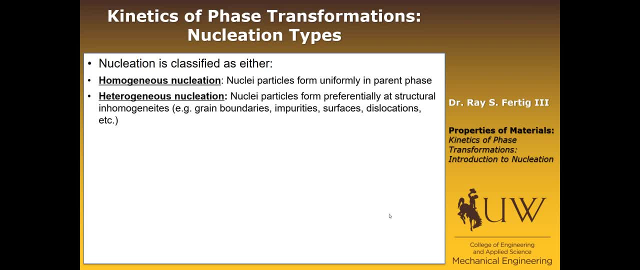 They just sort of form randomly in there. Heterogeneous nucleation occurs when the, the nuclei particles, are going to form preferentially at structural inhomogeneities, And we we've already drawn that a little bit in the the eutectoid transformation and microstructures for steel, where we said: 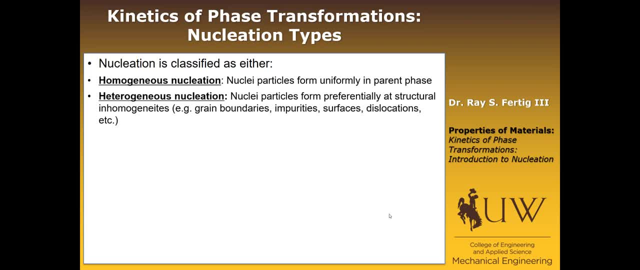 well, probably we're going to nucleate new phases at the grain boundaries and that would be a good example of heterogeneous nucleation, Or heterogeneous nucleation. Or they could nucleate other impurities, particulates, surfaces, dislocations, anything that causes basically a location of higher energy those particles can format. 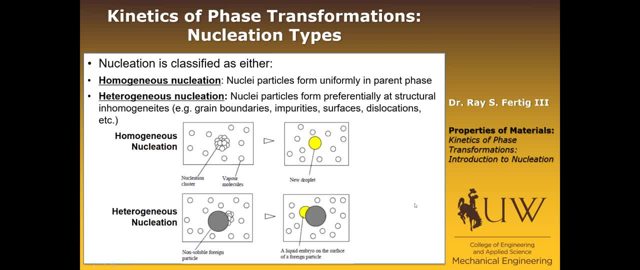 So those are the two classifications of nucleation. I'm just showing you a picture of that here. In the homogeneous case, we have to form a cluster of atoms, sort of in a random fashion, And then that this is. this is for vapor, but the idea is the same. 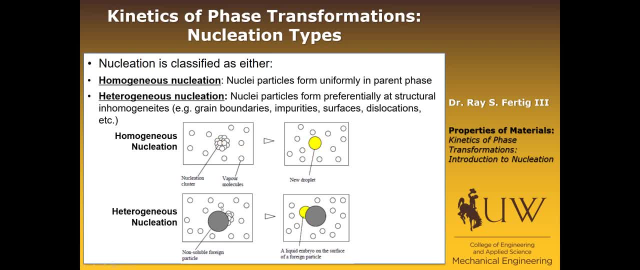 Then that acts as basically its own nuclei. that then can grow In heterogeneous nucleation there's some, we'll call it. in this case they're showing you a foreign particle, but some particulate, And the- the new phase, is going to grow on the surface of that particulate and then form the, the, the nucleus from which growth will occur. 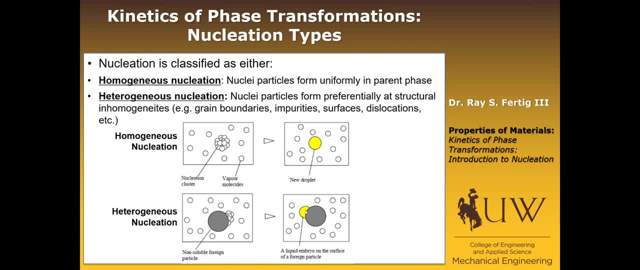 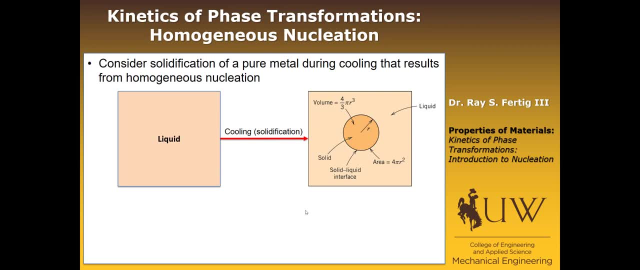 So those are the two types: homogeneous nucleation and heterogeneous nucleation. Okay, now we're going to get a little bit more technical. We're going to talk about the homogeneous nucleation. So we're going to talk about the homogeneous nucleation of a pure metal. 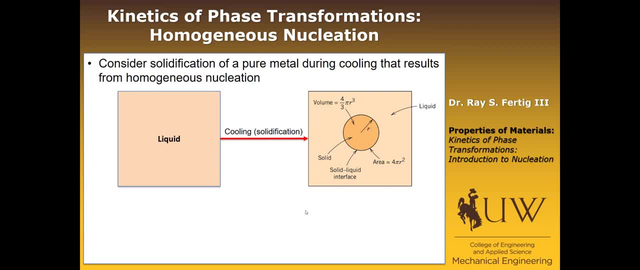 So this is going to be a solidification process- that during cooling, and it's going to result in some particle. So we want to think through the just the process and and try to understand the, the math that's behind it. 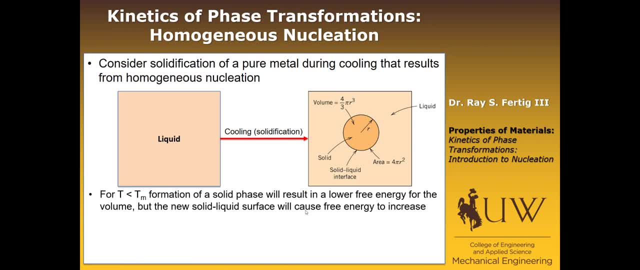 So obviously, for some temperature less than the melting temperature, the formation of a solid phase within the liquid is going to lower the free energy, at least within the volume where the transformation occurred. right, Because if it's below the solid phase then it's going to lower the free energy. 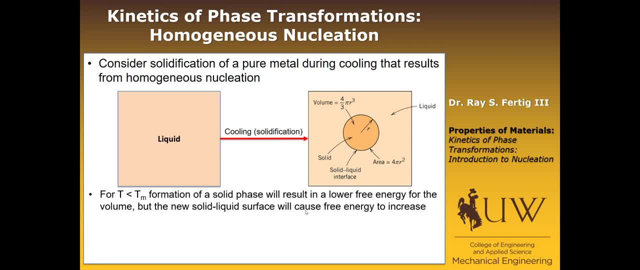 If it's below the melting temperature, then the equilibrium state is to have is to have the solid phase, not the liquid phase. But whenever we form that solid, there's going to be a new liquid-solid interface that's going to cause the free energy to increase. 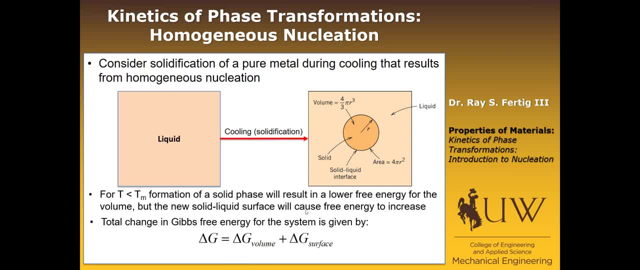 Okay, so we can write the total change in the Gibbs free energy for the system by saying that it's the sum of the reduction that we get in the Gibbs free energy, the volume plus the increase that we have from in the Gibbs free energy. 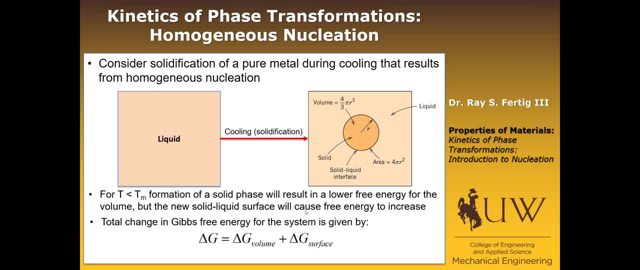 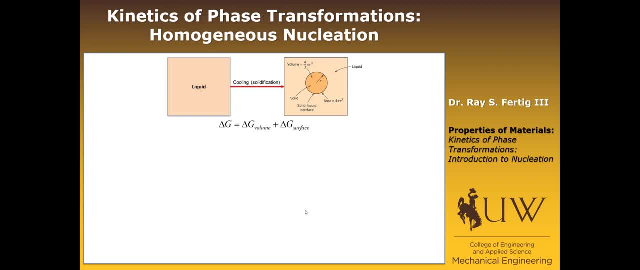 Okay, So let's go ahead and explore that just a little bit more. So this is just from the previous slide showing you what the total Gibbs free energy is in the system. And if we assume that that there's a change in Gibbs free energy per unit volume, we'll call it delta G sub V. that results just from the phase transformation process and the fact that it's it exists as a at a lower Gibbs free energy because it's we're now below the melting temperature. 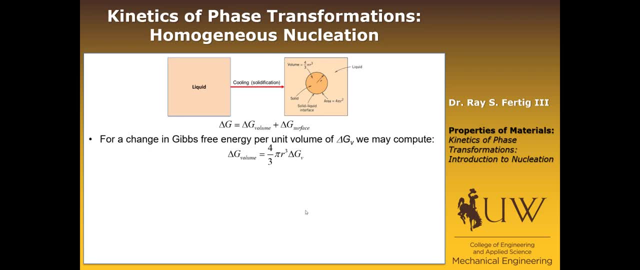 Then we can compute the total Gibbs free energy per unit volume. Then we can compute the Gibbs free energy change due to the volume changing to a solid, And that's just the volume of the particle. In this case we're assuming a spherical particle. 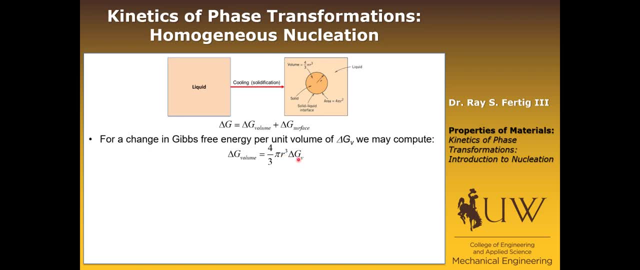 So the volume of the particle is four thirds pi r cubed times delta G sub V, which is just the free energy change per unit volume because of the phase transformation. Okay, so just remember that because delta G sub V is less than zero, right, it reduces the Gibbs free energy. 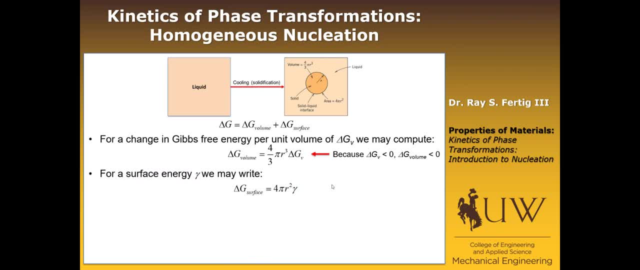 Then delta G sub V is less than zero. Okay, so for the surface energy gamma we may write that the delta G of the surface here is going to be equal to the surface area of the of the particle, which is four pi r squared times the the the surface energy gamma, which is actually a per unit area quantity. 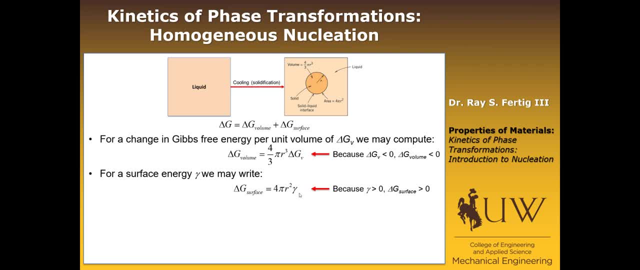 And then, because gamma is greater than zero, then delta G of the surface is going to be greater than zero, And then we can write that Again. going back to this top equation, here we can write again that the total change in the Gibbs free energy can be written in this form here: 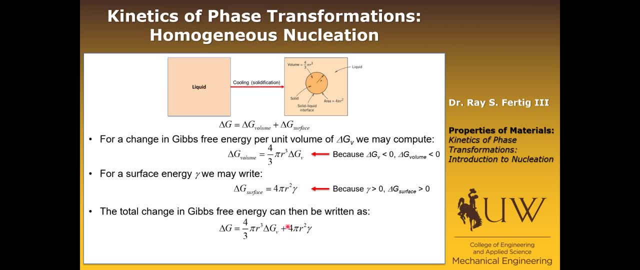 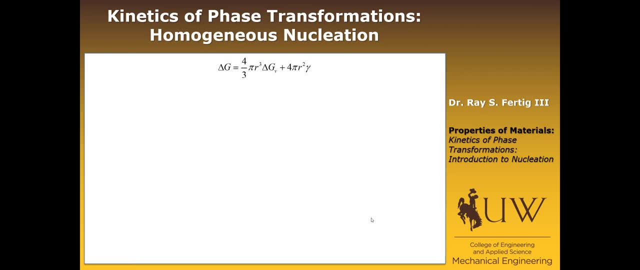 where we have the contribution from the volume and the contribution from the surface. So that's the total change in the Gibbs free energy. Hopefully that's pretty straightforward. So let's begin with that And let's just ask some basic questions about what we could expect from this equation. 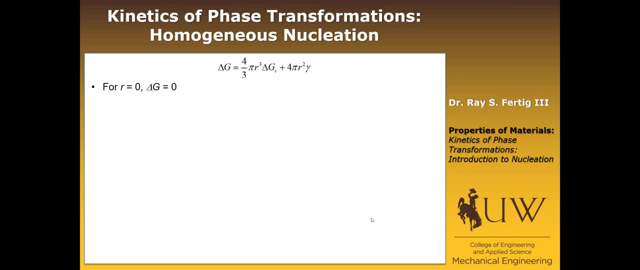 Well, obviously, if R equals zero, then delta G equals zero. right, That's straightforward. You can look at the equation and plug that in. If R is very small, then R cubed is going to be much, much less than R squared. 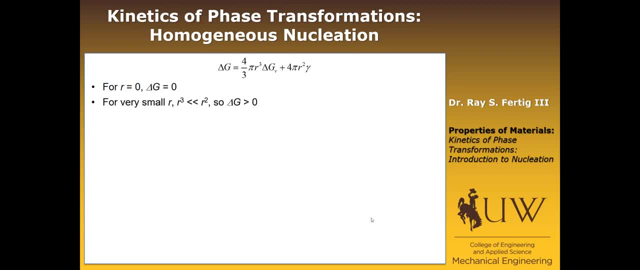 So delta G is actually going to be positive initially. So we start out with delta G zero, We go to delta G is positive And that's because we're actually increasing the energy due to the surface energy And the energy reduction we get, for the volume isn't sufficient to overcome that surface energy. 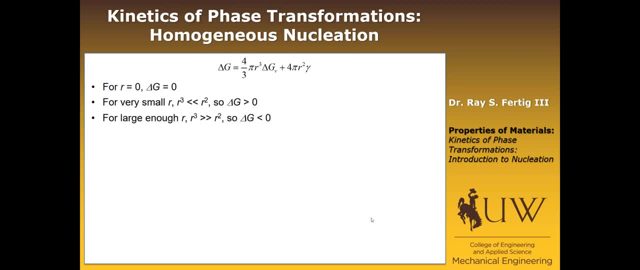 But at some point for R large enough, then the R cubed term, or the volume term, is going to dominate the R squared term. So delta G goes back to less than zero. What that hopefully says to you is that there must exist some maximum in the Gibbs free energy delta G. 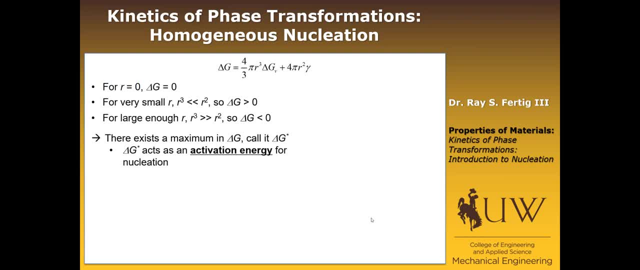 Let's call it delta G star, such that delta G star is going to act as an activation energy for nucleation. Okay, so here's the diagram. This red curve is the Gibbs free energy that's a result of the surface. This blue curve is the Gibbs free energy that is a result of the volume. 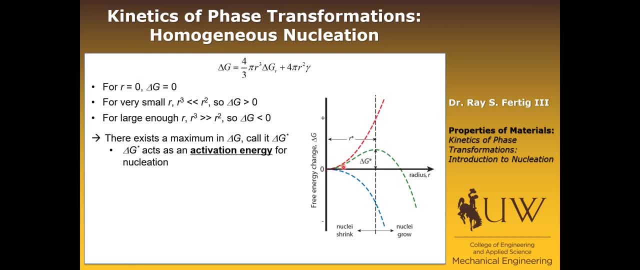 And if we add them together, we end up with actually something that begins at zero, ramps up to some value and then dives off as the radius gets larger, And then the radius gets large enough. Okay, so we're going to try to look at how we can compute this delta G star. 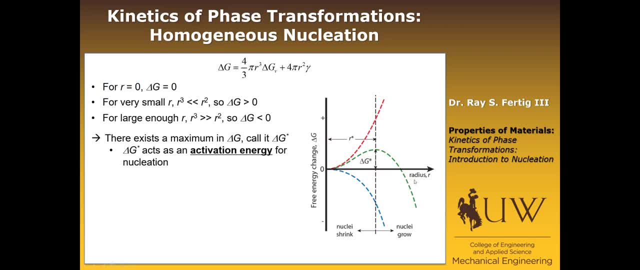 because that's how much energy we have to overcome to actually create a particle that's stable. The radius at which that occurs- so this is R star- is going to be called the critical nucleation radius, And it might be tempting to say, well, maybe the critical radius should be. 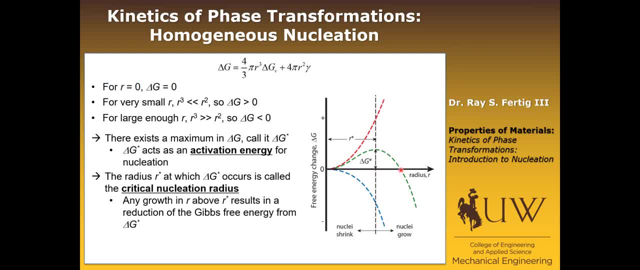 where delta G equals zero. but really what we want is we just want it such that any increased growth from R star is going to cause a reduction in the Gibbs free energy of the system. So we just need to figure out where R star occurs such that any growth above there is going. 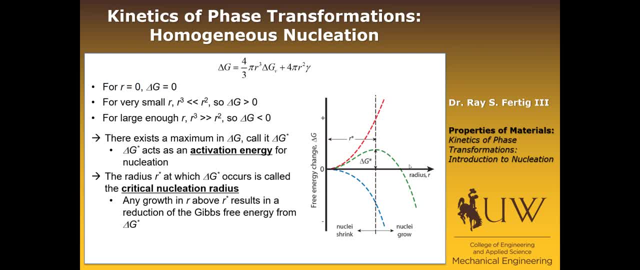 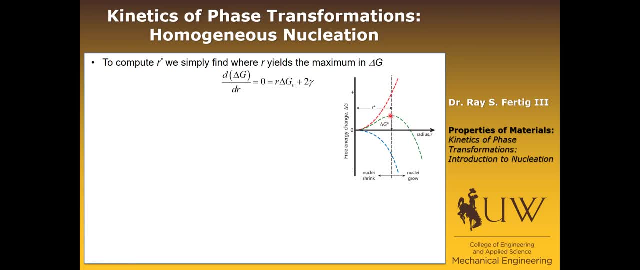 to allow the particle to grow stably. Okay, So how do we figure out that? Well, we know that R star occurs when delta G is a maximum, And so we just need to figure out where delta G is a maximum. We do that by taking the derivative with respect to R and setting it equal to zero. 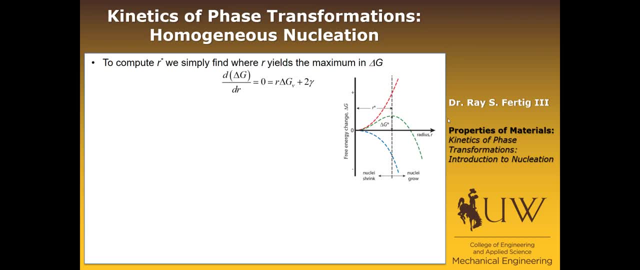 We end up solving. you can do a little bit of algebra on it and end up seeing that it's just R, delta, G, V plus two gamma. So then we can easily solve that for solve for R, which gives us R star. 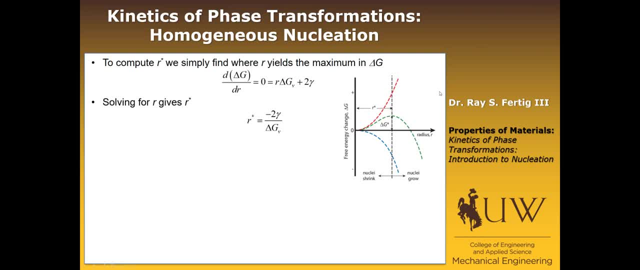 and see that R star is going to be negative two times gamma divided by delta G V. Okay, We can then use R star to compute delta G star. Delta G star then ends up being 16 pi over three times gamma cubed over delta G V squared. 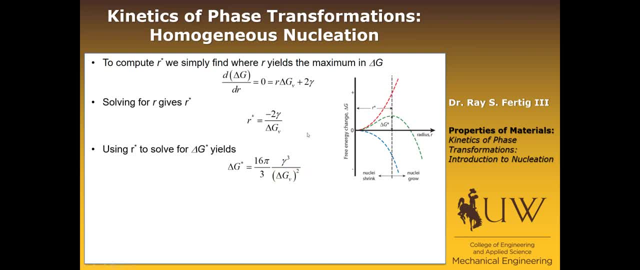 And this term is going to become important in the next lecture, as we talk about what controls the change in the volume term of the Gibbs free energy on a per unit volume basis. That will be the focus of our next lecture. But the upshot of all of this is that, in order to create a stable nuclei from which to grow, a new phase